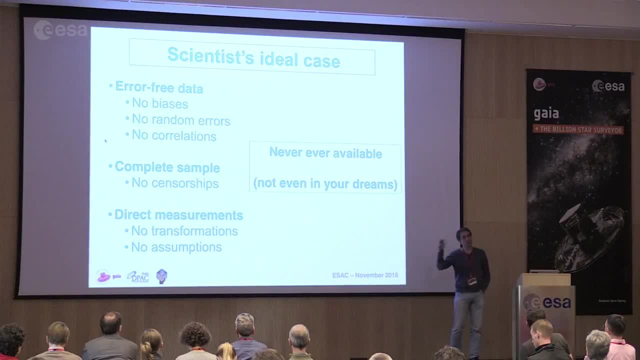 of the quantity we are working with and not a measurement of another quantity which we have to transform to our quantity to work with And no assumptions about those transformations. So we will never have that, Not even in our dreams. We dream with having error-free data. 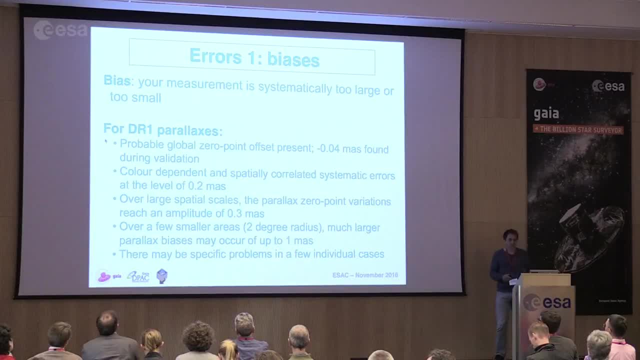 because this is simply not possible. So Leonard has been discussing about biases. Biases, essentially, when your measurement is systematically too large or too small with respect to reality, a reality we would never have access to. For the DR1 parallaxes, as already been mentioned, we have some zero. 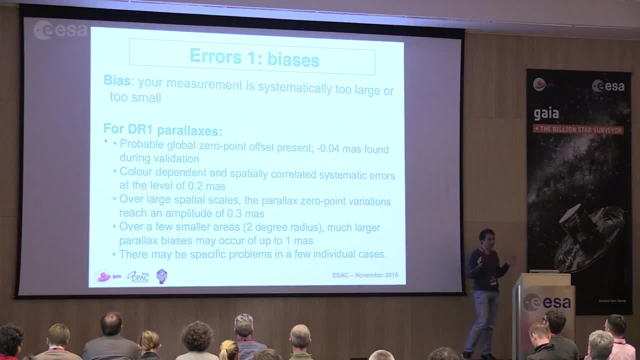 points. So globally the Gaia parallaxes are slightly too large, slightly too small And they are not a problem. From the validation work we have found possible value of minus point zero four. So parallaxes are slightly, have to be slightly corrected. I'll discuss about that later, But this is. 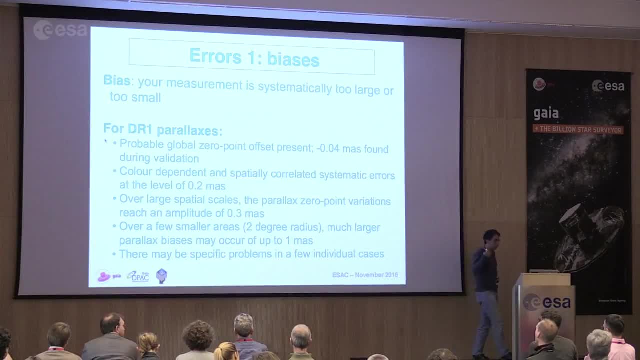 the order, point one, no more. There are also color dependent correlations. sorry, color dependent and spatially correlated systematic errors at the level of two milli point, two milliac seconds, And overlap you large scales, we have to assume that there could be. zero variations in this zero point. globally This is small, but locally could be as large as 0.3 or more, Because in a few small areas of a few degrees these variations of the zero point can go up to 1 milliac second. 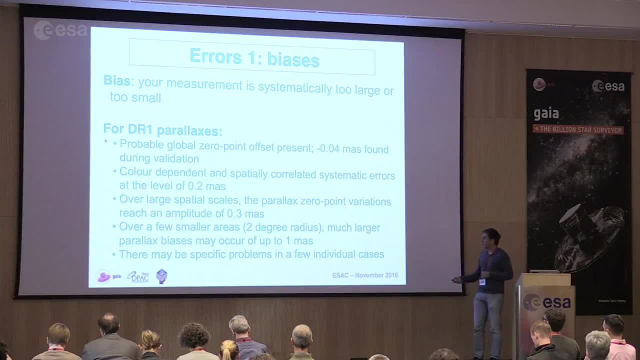 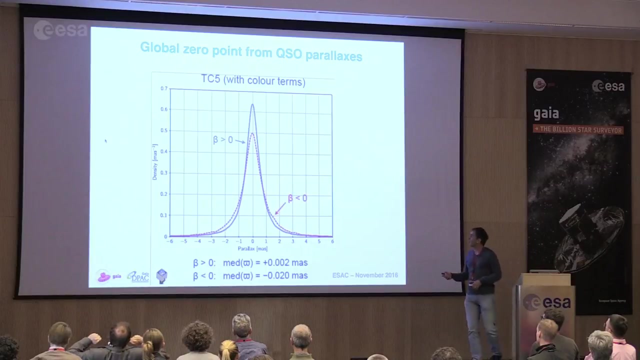 More about that in a moment. And in addition to that we may have specific problems in a few individual cases. So specific biases for specific objects. All this sounds very, very bad, but it's not that bad. OK. this is an example of the estimation of the zero point. 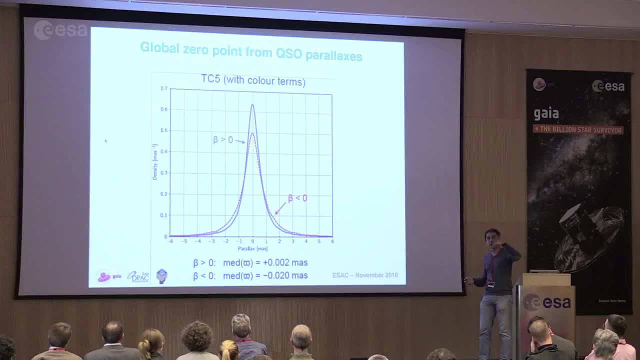 from QSOs. It's essentially similar to the figure that Leonard has presented, but presented in a different way, for northern and southern ecliptic latitudes. As you see, for quasars the number is quite small, And this is from the CFITs. 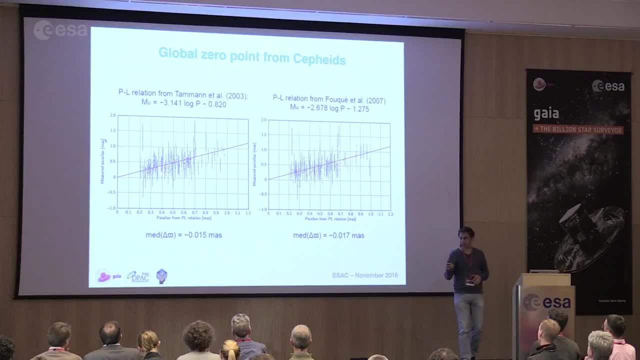 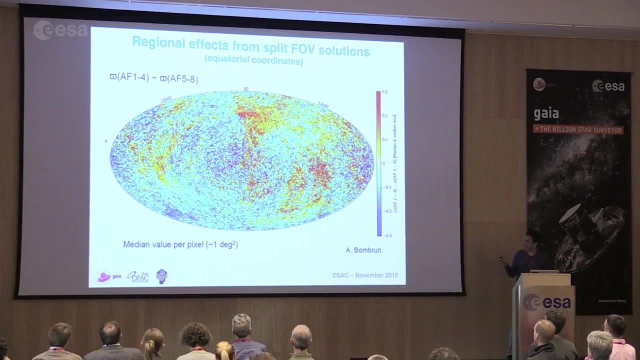 We are also getting very small zero points. globally OK, but if you go zonally, in regions, this is already seen. Leonard has already shown this split field of view. So comparing half of the focal plane with the other half. So, as you can see, depending on the region, 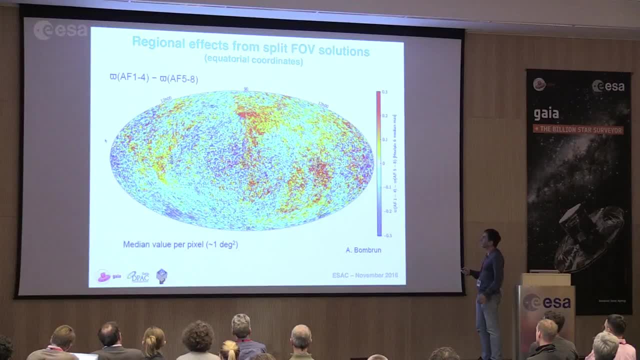 you might have variations between one solution or the other of 0.3 in one sense or the other. So this is it. This is the level Our parallaxes can be, depending on the region. slightly too high, slightly too small. 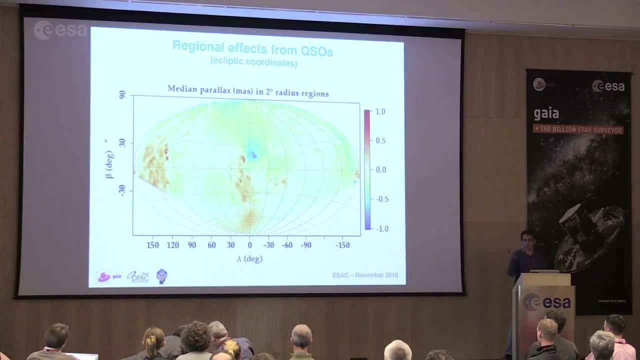 This is another figure not shown before. This is from the validation work, from the CU9 work package devoted to validation. Sorry, I'm making a lot of noise here. Maybe take off your badge. Oh, Let's see a bit better, OK. 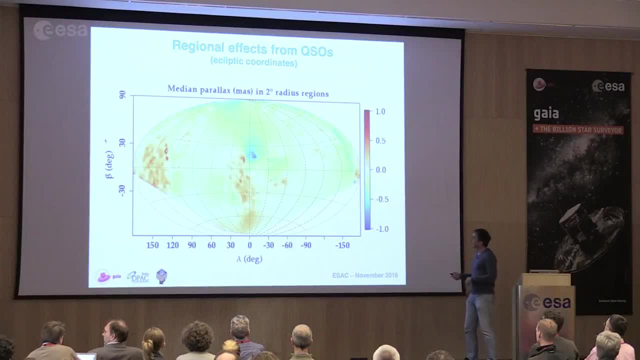 This is a comparison. This is a comparison with quasars, showing that originally, for instance, here minus 1 or around here plus 1, we can have a systematic local zero point of the parallaxes that can be somehow large. But for most of the sky this is good news. 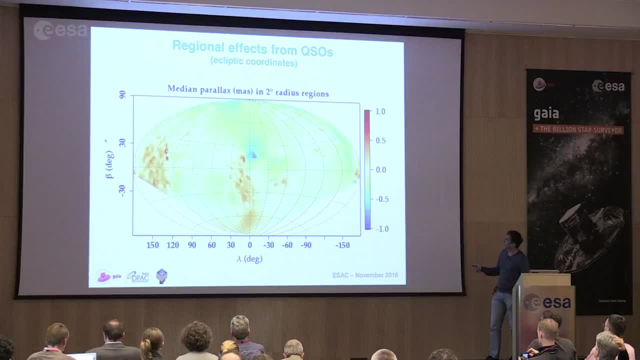 For most of the sky. the values are again very small, But be aware that if you happen to be in one of those regions, you might be unlucky And your parallaxes might have a little bit more. It's a bias, a significant bias. 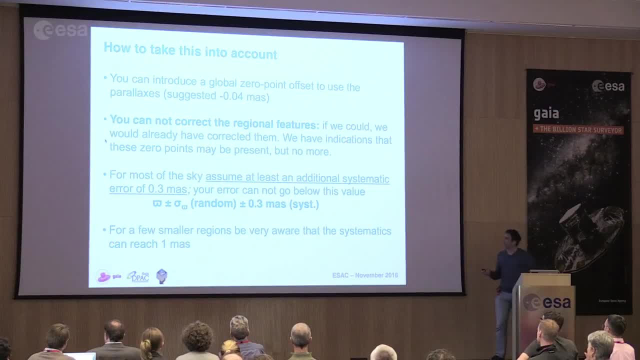 OK, What can we do about that? I would say first, it is OK to not introduce any zero point correction, Or, if you wish, you can- This is a value suggest. You can introduce a very small one, But at this point we cannot say what is better. 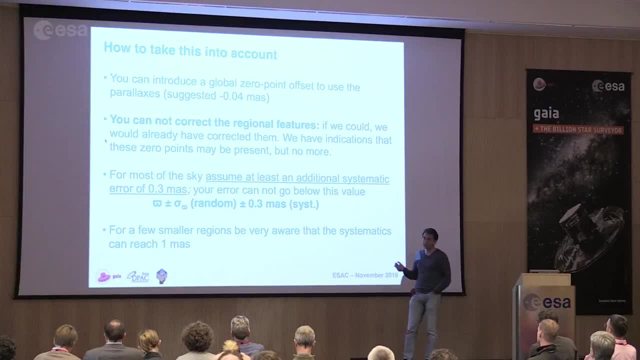 We suspect this is a value which should be subtracted. But if you don't do that, it's equally better. Again, with the R1, we cannot do better than that, But if you want to play on the safe side, it could be OK to subtract this value from all your parallaxes. 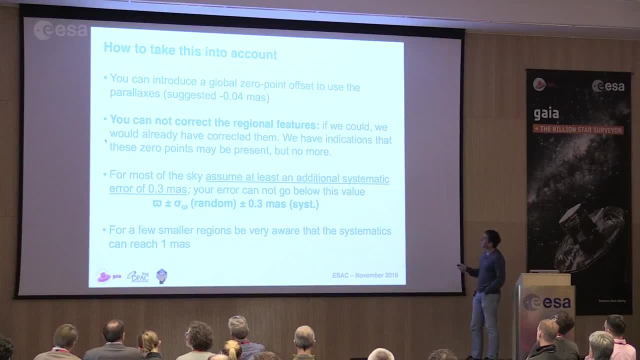 But what you cannot do is correct the regional features, As Leonard has already said. if we could do that, we would already have done that. Do not go to the previous map, say, oh look, I am in this region. Let me add or subtract 0.1 milliac seconds to our parallaxes. 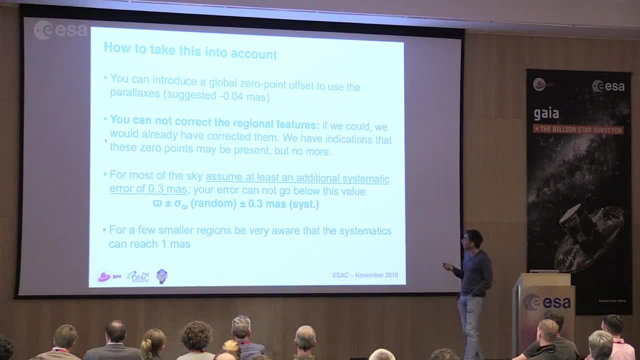 Because you could even do things worse. You could make things worse In addition, for most of the sky. you have to be aware that you have to assume an additional systematic error of about 0.3.. Your error cannot go below this value. 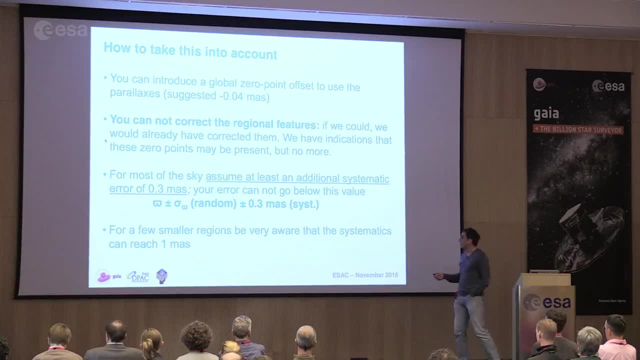 So, as pointed out in the paper describing the release, your parallax has to have the error given in the catalog, But you have to take into account 0.3.. OK, 0.3, additional 0.3, a systematic one. 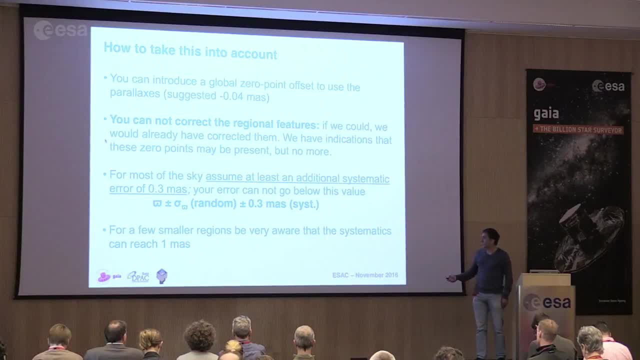 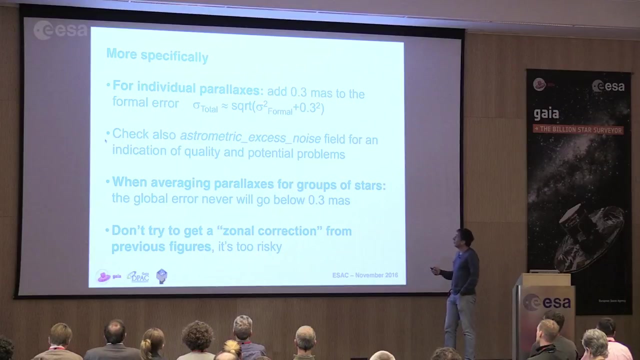 How to treat that In a moment, And be aware that for those small regions that I have shown in the previous map, you can have even larger systematic errors. So, more specifically, when you are using a single individual parallax, OK, the suggestion. 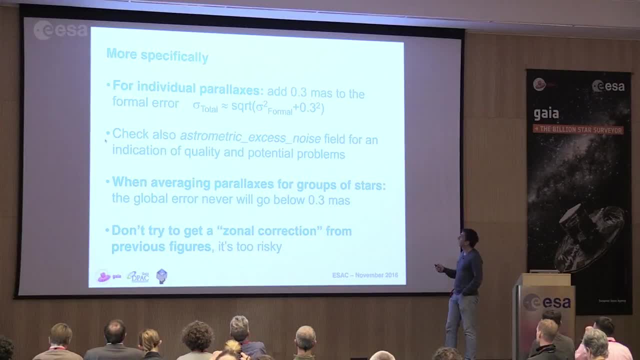 is to take the formal error, the one given in the catalog, and add 0.3 in a quadratic way, proper way. so you have a total individual error which is larger by this quantity with respect to the one given in the catalog. 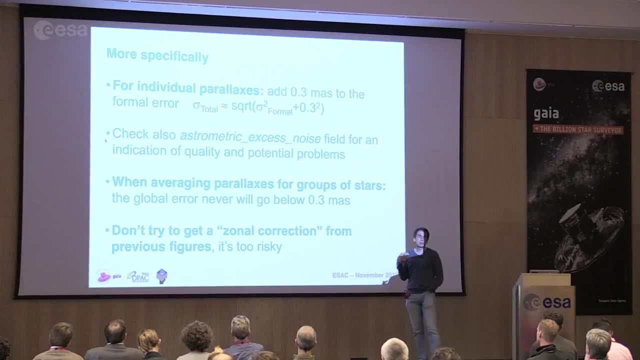 This is to play in the safe side. Probably we are overdoing it. The formal errors already contain some margin and this is a kind of worst case. on average It could be even a bit small in some specific regions, but on average for all this sky. 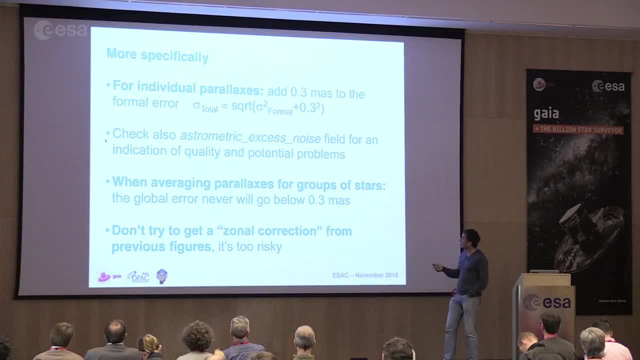 this is overdoing it a little bit. But if you want to really be on the safe side, do not simply take the formal errors in the catalog, add this quantity. For example, you take the formal error of 0.3 in the catalog and you add 0.3, you give 0.3. 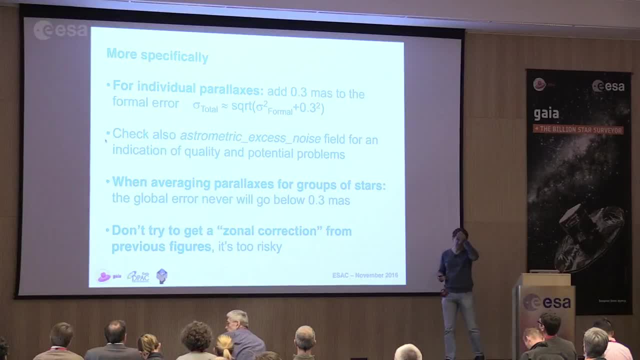 in the catalog may be one saved error, So the common error could be 1: 1, in the case of the more popular model, 0.3, or 1: 1, or 0.3. So this can be that one. 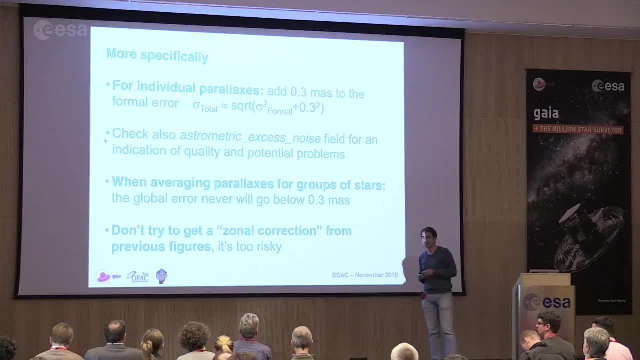 And this is the one here. that's the one that I'm telling you about in the show window, with some more formats, And that's also one that I want to add, but this is not necessarily the most useful one: 0.25 milli-arc. second, 0.5, okay, 0.25, 0.25. so we do get below the 0.3, okay, but for 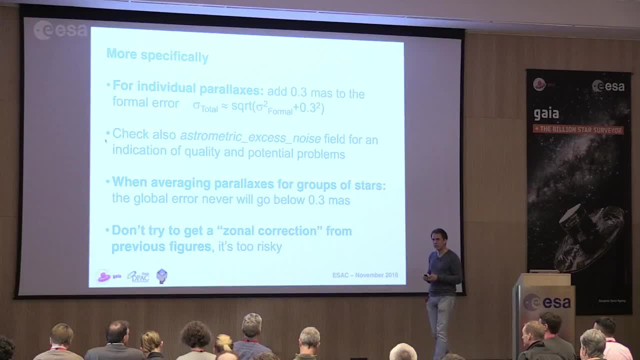 clusters. so when I, when I compare the Hipparchos cluster parallel axis with the TIGAS cluster parallel axis, I need an excess noise of the level of 0.25 milli-arc second to make the two sets agree. yeah, not 3 milli-arc seconds. 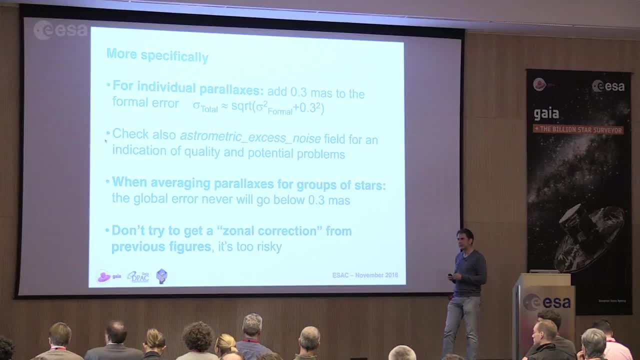 so we do get below the 3 milli-arc, the 0.3 milli-arc seconds. okay, this is a kind of worst case, yeah, but if you say then the global error will never go below the 0.3 milli-arc second, I think it does. okay. again, I was getting here. 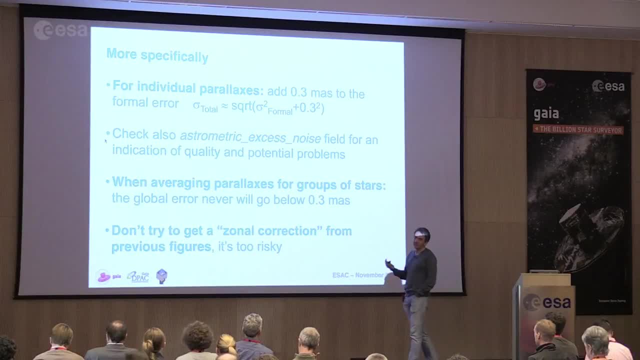 again we are playing it safe. okay, probably in the cluster paper I will show that it's down to 0.25, but the cluster paper is specific to the TIGAS cluster parallel axis and the TIGAS cluster parallel axis is down to 0.25. 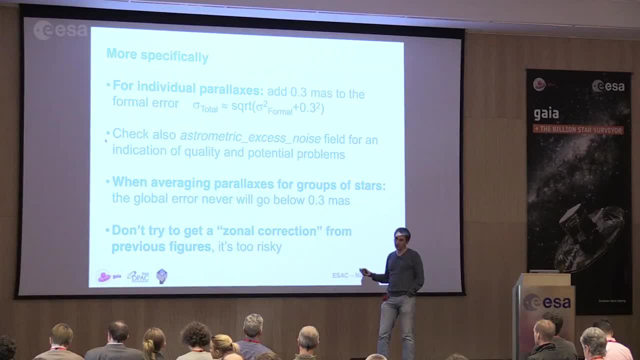 regions of the sky, so, and the rest of the sky, you can get. you can have cases where it's worse. so for a global recipe, a global advice on what to do if you don't want to take more specific advice. does not contain the word never okay. 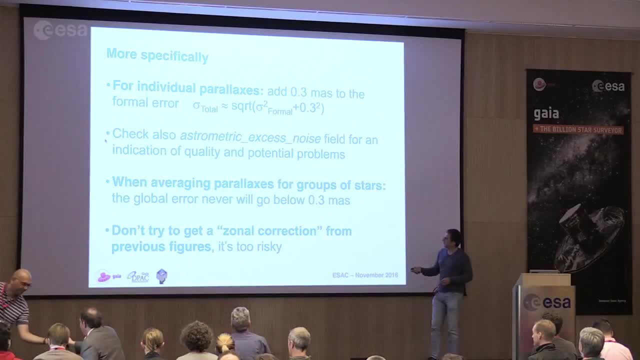 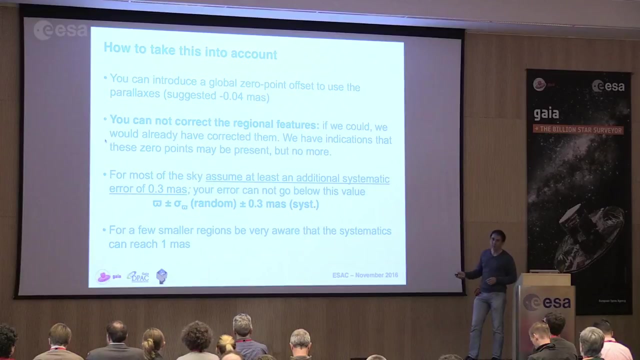 should never go below 0.3. the idea, what I wanted to stress here, is that if you take a group of stars and you average the parallel axis of those stars, you will be limited by the systematics you will. this will average out we at the square root of n, but this will not. so you can. reduce, when averaging groups of stars, this contribution by adding more and more objects, but this will stay there. so the suggestion is to keep as a global recipe a minimum error of 0.3 mass when you ever are averaging stars, if you are doing a specific work. 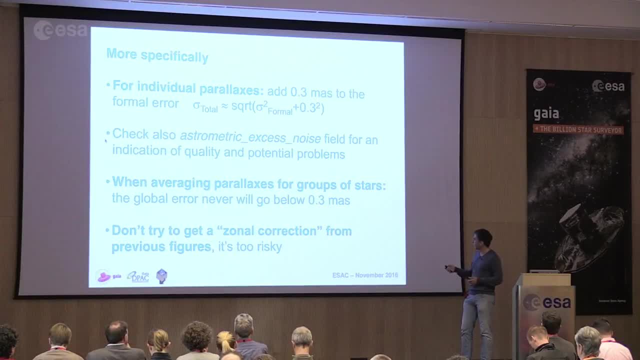 like floor. okay, you, you will know better. but this general safe recipe, keep at least this point three months when averaging parallel axis. and again, do not try to get a zonal correction from a previous figure, because it's too risky. you may be making things worse than they are. okay for proper motions and 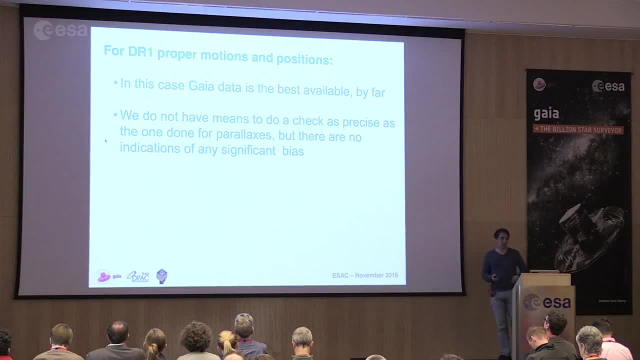 positions. in this case the Gaia data is best available by far and we do not have the means to check, to do checks validations as precise as the ones done for parallaxes. but in the margin of error, we have no indications of any significant bias. 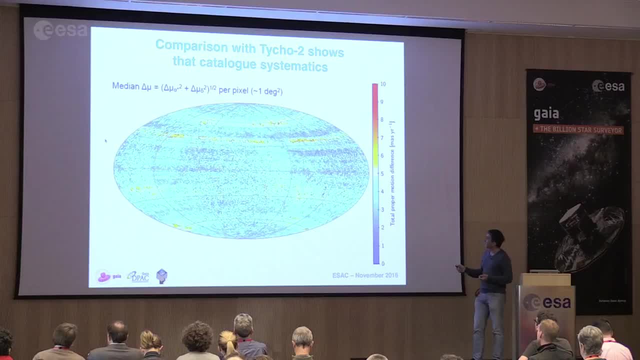 When you compare with TYCO2, this is what you get. but those zonal fringes, those frames, well. so those strips are likely, or almost surely, due to TYCO2 and not to Gaia. So, for proper motions, I think it's safe to assume that we do not have significant bias. 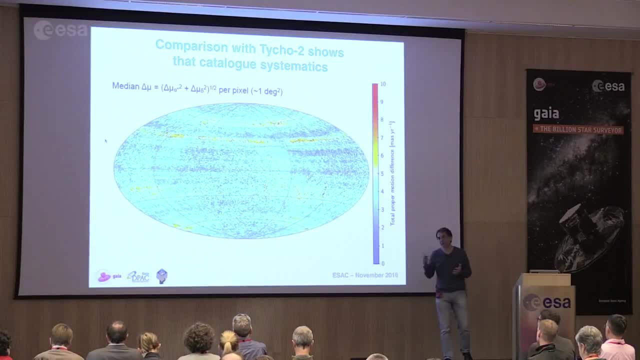 but be a bit careful about that and, as a general message, wait for DR2, where things will be even better. One thing I forgot to add here is about positions. Positions are also very good. No special indication of biases, except maybe some when comparing with the ACRS, some residual rotation, but very small. But here the problem would be, that if you want to compare positions with other catalogues, you will have to do an epoch change. You can properly do that when you have proper motions, but then you have to propagate the errors accordingly. 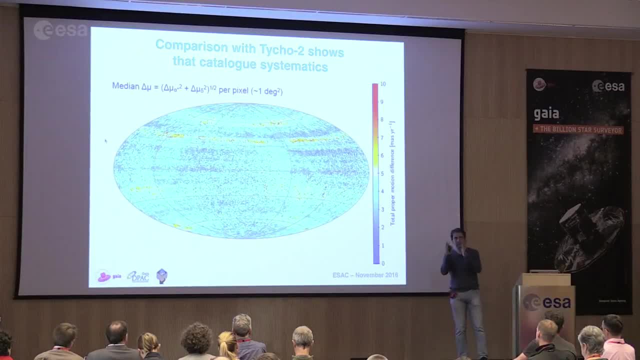 And when you do not have proper motions You cannot properly propagate to another epoch. So you will have to take into account a larger error when comparing your position, Gaia position, with another position. But probably Gaia position will be far better than any other position from ground catalogues. 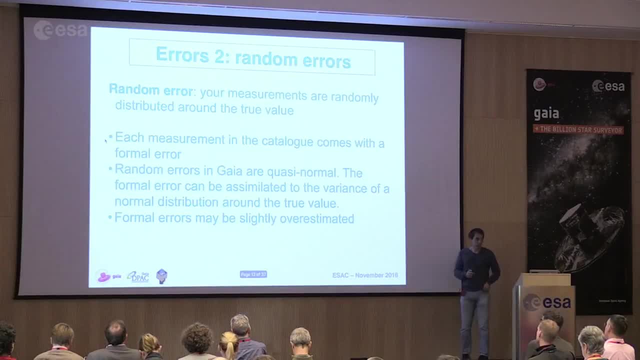 HST will be a different issue. Okay, random errors. Random: yes On proper motions. can't yield On proper motions. can't yield. Okay On proper motions. can't yield. Okay On proper motions. can't yield. Okay On proper motions. can't you look at the quasars which you expect, for physical reasons, to have? 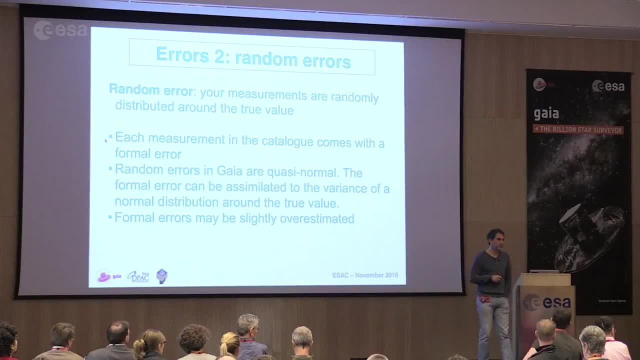 near zero proper motion. Yeah, yeah, That's like 500,000 million sources. The problem with quasars is that in the solution- correct me, Leonard, if I'm wrong- it was assumed that they have zero proper motion In the auxiliary solution but not in the main solution. was my understanding? 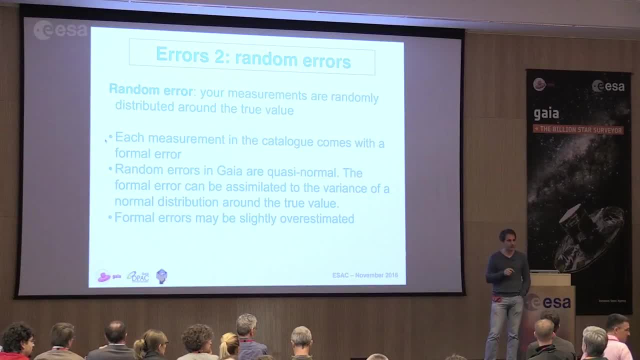 Yeah, You mean okay. Can you go to the main solution, not the auxiliary, and look at proper motions of quasars, Mm-hmm. Not enough, Okay, For random errors. you know your measurement is randomly distributed according to some PDF around the true value. 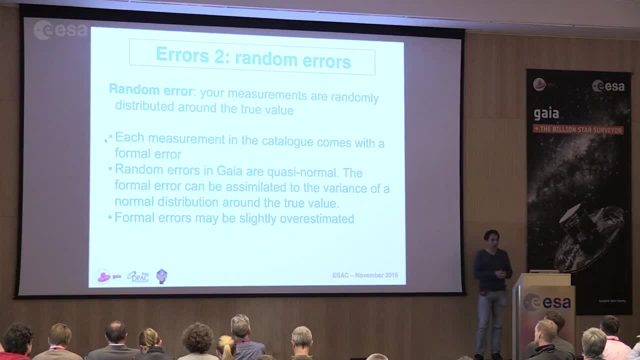 So each measurement in the catalog comes with a formal error and those errors for indicated by Leonard for the astrometric solutions are quasi-normal. So the formal error can be assimilated to the variance of a normal distribution around the true value And, as already discussed again, the formal errors might be slightly overestimated. 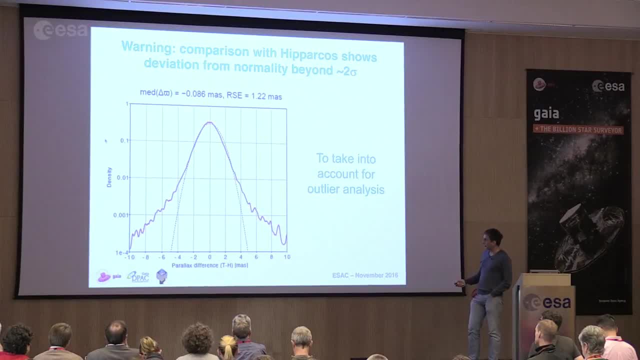 Some considerations. This is a comparison of TIGAs minus Hipparchos parallaxes. One would expect this comparison to follow this line. Okay, If both errors were normal, But as you can see, there's a deviation at the tails from normality. 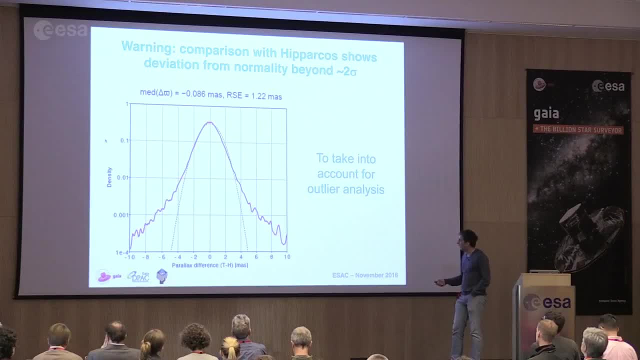 Well, this is TIGAs versus Hipparchos. You cannot be sure why this deviation or where this deviation come from, Hipparchos or TIGAs, But take into account that it might happen that beyond two sigmas there are more objects. 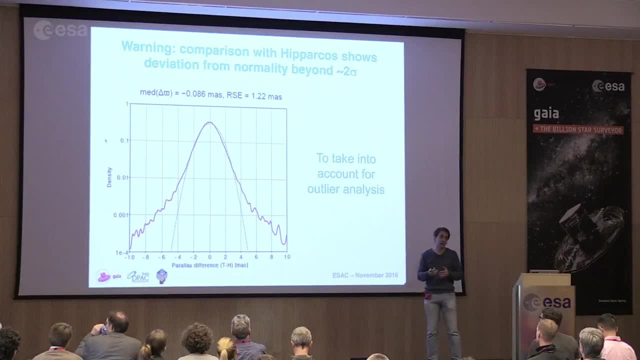 than expected from a pure normal deviation. So you will have outliers if you assume that the distribution of errors is fully normal. So objects that are beyond what they should be. But again, this is Hipparchos versus TIGAs. Could be one or the other, or both. 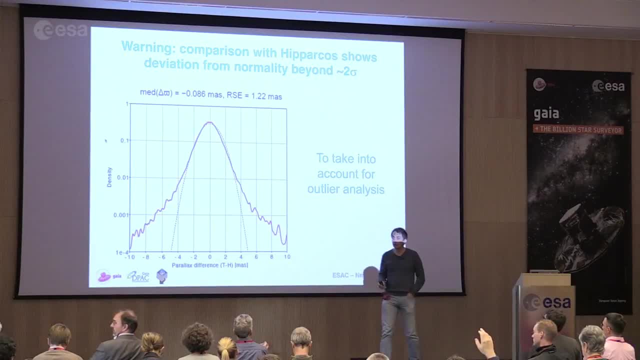 But at least take into account that you can have some outliers. Well, two questions. Has this been selected on solution type in the Hipparchos data? This figure is from Leonard Leonard. I have to check the paper to answer the question. 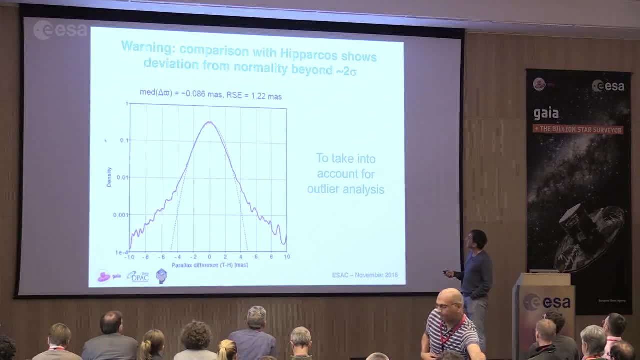 If I am able, values that are larger when you expect from a normal distribution, either from astrophysical, 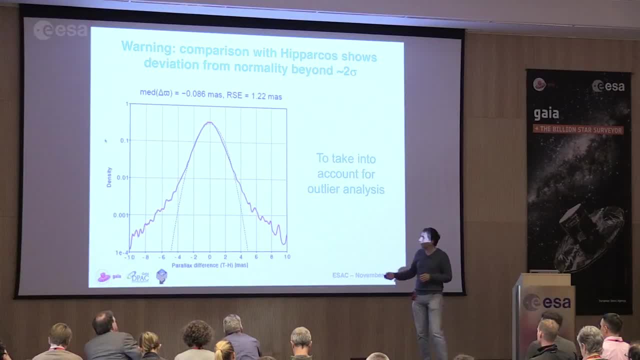 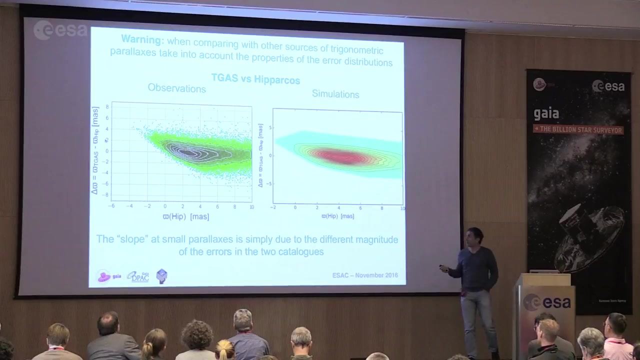 reasons, or either from problems in the solution. Just a small one. There are not many, but be aware when doing some very extreme analysis that extreme cases might be more frequent from what you would assume from a normal distribution. Another warning is about the usage or comparison of data. 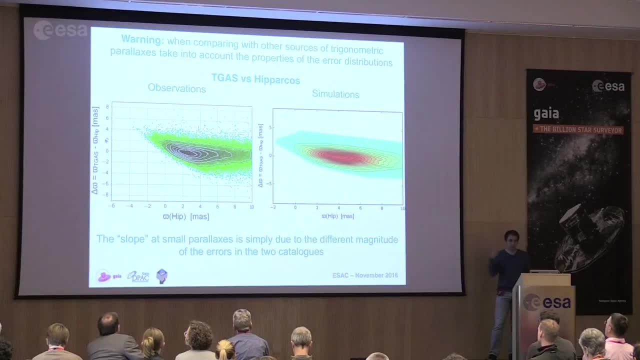 The warning is about when comparing parallaxes from TIGAs with other sources of parallax. This is an example. This is on the horizontal axis. is Ipacos value of the parallax versus the difference between the TIGAs parallax and the Ipacos parallax? 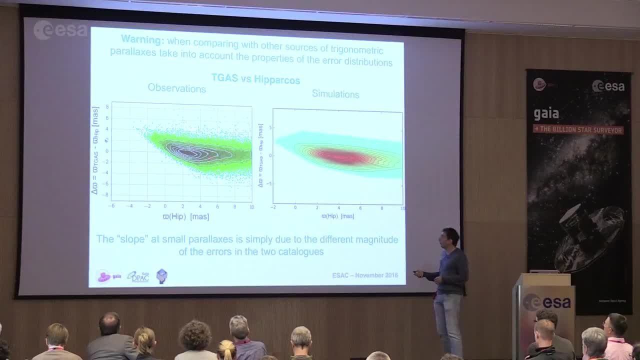 The distribution has this shape, One could think that there's some kind of bias for these small parallaxes, while in fact, this is exactly what we're looking for, Exactly what you expect from the fact that the error in Ipacos is larger than the error. 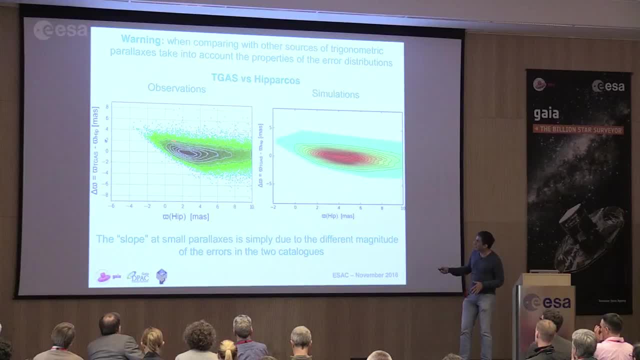 in TIGAs. This slope here, this apparent deviation versus large values here is exactly what you would expect. In fact, this is a simulation with similar parameters and their true data and you can see a very similar effect. You can see this deviation versus large values here. 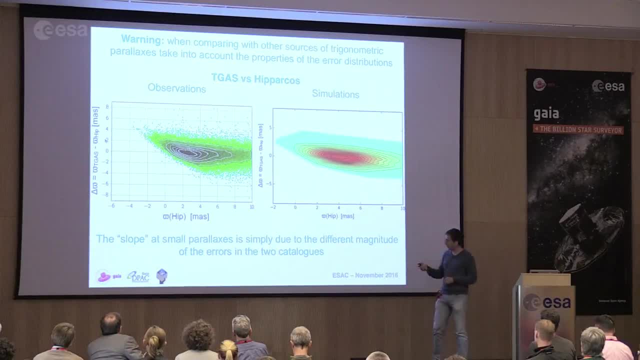 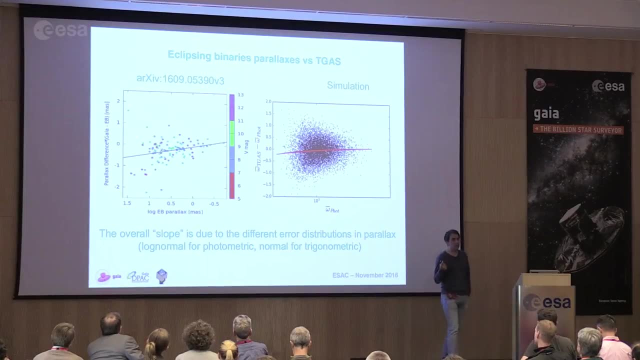 The warning is because If you are not careful, If you do not take into account the properties of the error distribution, you can make mistakes. and this is a suggested example. This has been published in our archive. This is a comparison of parallaxes from ecliptic binaries versus the difference between Gaia. 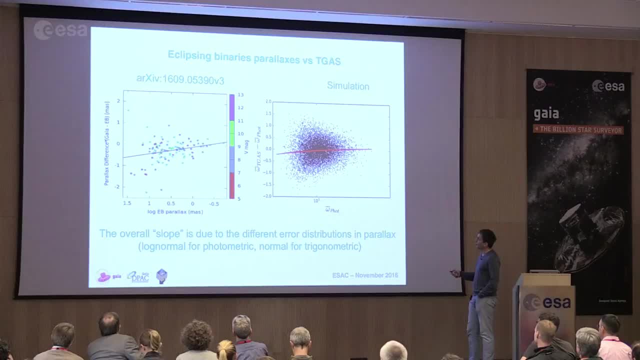 or TIGAs and ecliptic binary parallax, and the author suggests some systematic or detection of some systematic effect from the fact that this comparison has some slope, While a simulation of the same situation gives a similar slope just because of the properties of the distribution of the errors. 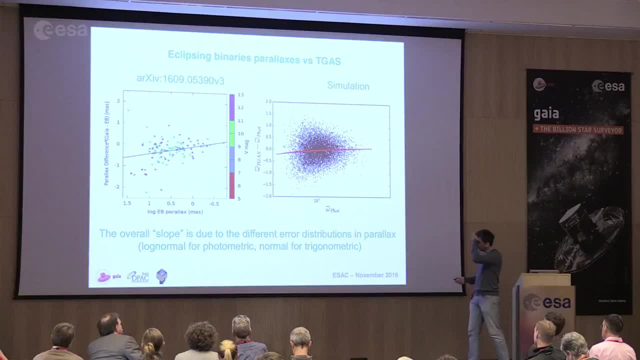 In the case of the Ipacos parallax, the error is normal, while for photometric parallaxes, or parallaxes coming from this ecliptic binary method, the distribution is rather log normal. So overall, the different distribution of errors gives an effect like this: 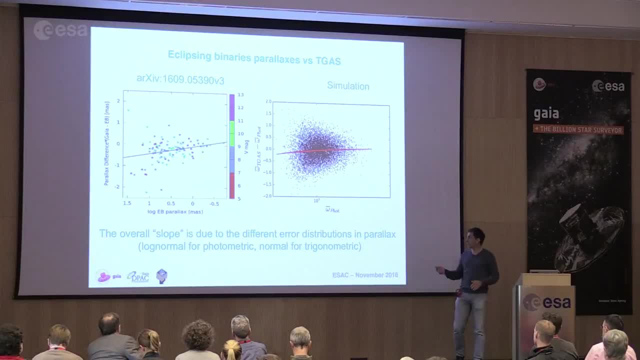 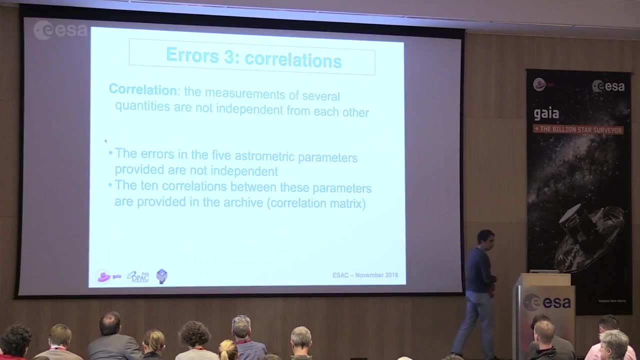 So this is a warning on this- On the comparison of sources of parallaxes, especially in this case photometric versus trigonometric parallaxes, Correlations: We have correlations in all quantities. Correlations is when a measurement is not completely independent from another. 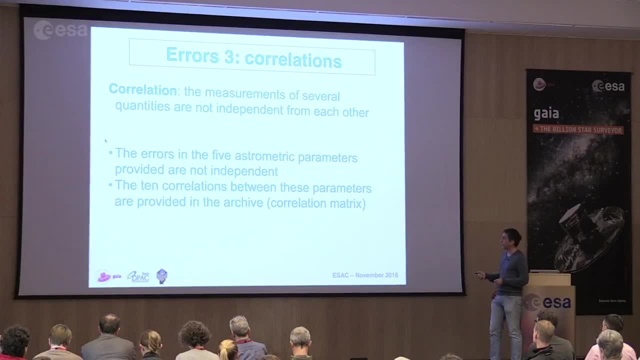 The five astrometric parameters have correlations. They are not fully independent, They come from a common solution And the ten correlations between these parameters are provided in the archive. It's fields called like parallax, declination correlation, et cetera, et cetera. 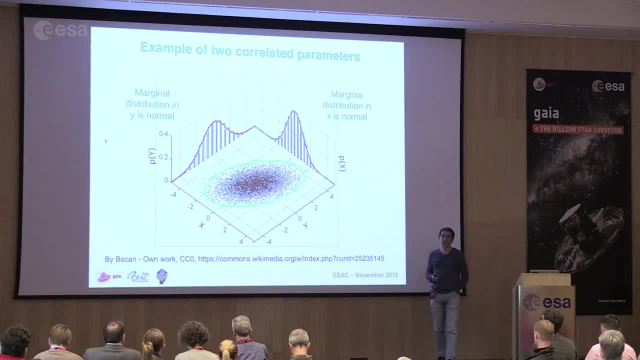 Essentially, the correlation matrix is given How to interpret this. So this is, in two dimensions, an example of correlation. The quantity Y, when taking alone, is normally distributed. Quantity X, when taking alone, is normally distributed. And when you look at them together in this plane, you see that the distribution of the 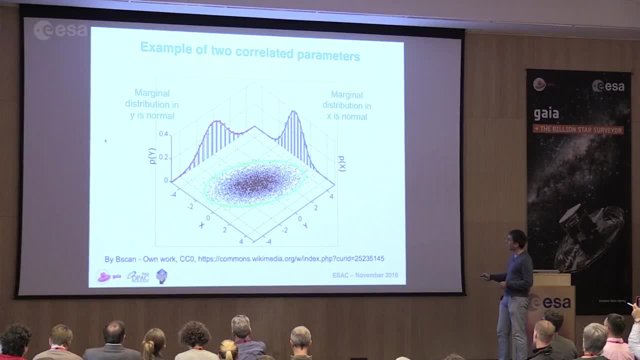 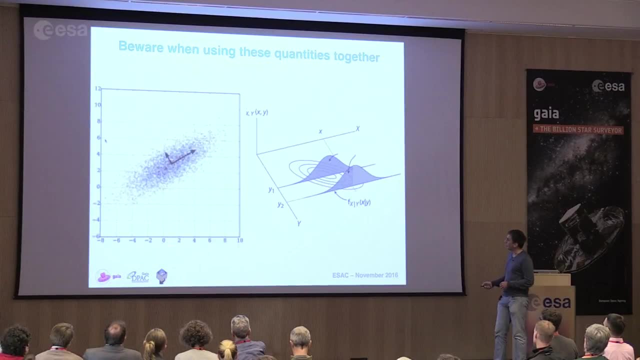 point. the joint distribution is an ellipsoid which has an inclination When this happens. a situation like this means that if the deviation of measurement in X is positive, the deviation of the measurement in Y tends to be also positive. So one error is not independent of the other. 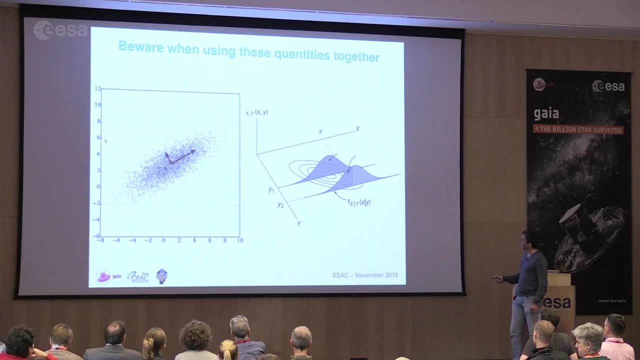 So, for instance, If you look at this plane and you see that the distribution of a point, the joint distribution, is an ellipsoid which has an inclination, measurement in Y is truly has a net zero error. the maximum in X has a distribution exactly distributed around the true value. but if the measurement in 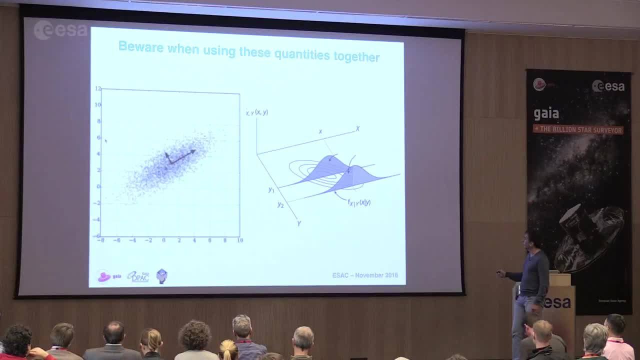 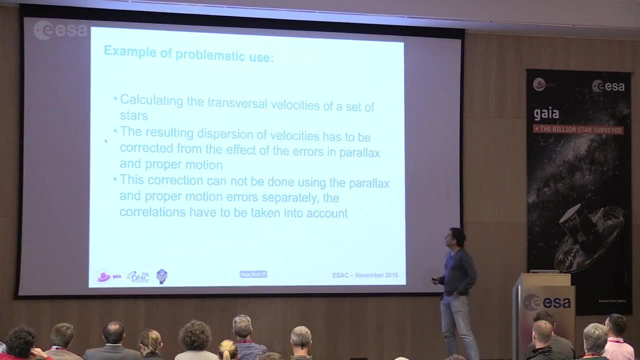 Y. it's larger than the true value. your measurement in X will be distributed around also larger value. this has to be taken into account, especially when you use more than one astrometric parameter at the time. typically, the case where this is relevant is calculating transversal velocities or space. 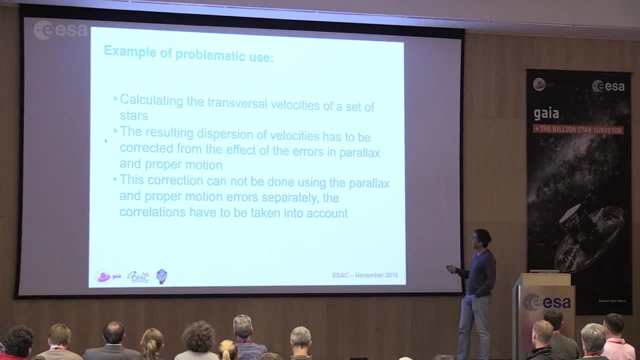 velocities. if you have a radial velocity for a set of stars, the dispersion of velocities that you get will be the composition of the true dispersion of velocities plus the effect of the error. so to obtain the intrinsic dispersion of velocities you have to subtract the contribution of the observational errors. 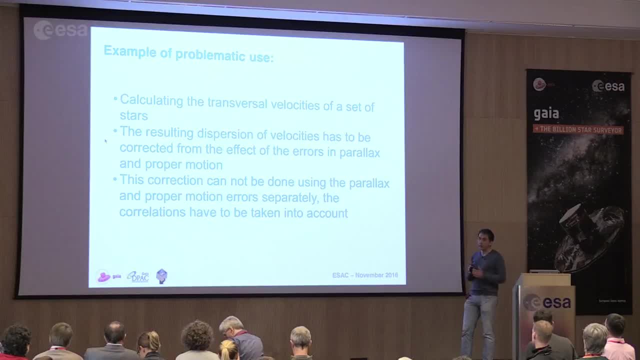 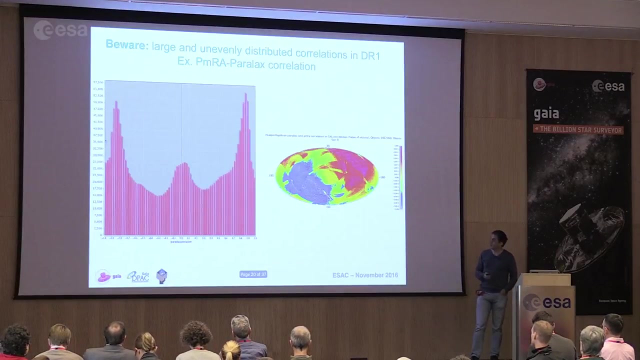 but to do that you have to take into account that at the error in distance and proper motion in alpha and Delta are correlated, otherwise you will be overestimating the contribution of the, the errors, into the dispersion. so this is warning and example, and taking to account that in DR1 the correlations 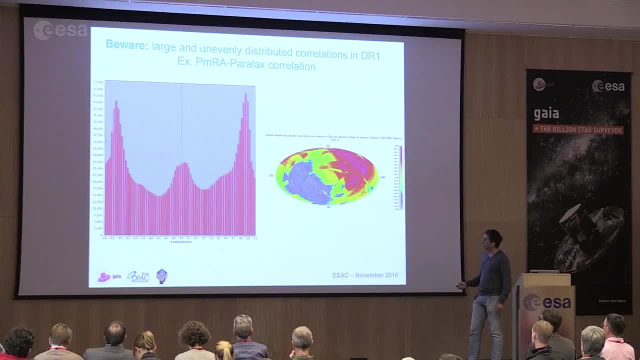 might, might be large. as you can see, this is the parallax proper motion, right ascension correlation in. one would like or would expect the correlation to be around zero, but notice that they're a large fraction with very large correlations. Even worse, they are spatially distributed in a very inhomogeneous way. Here you have. 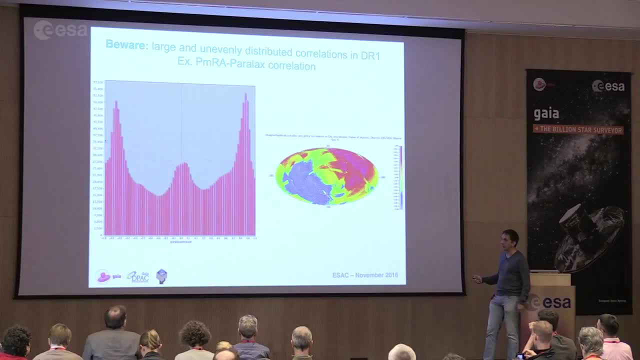 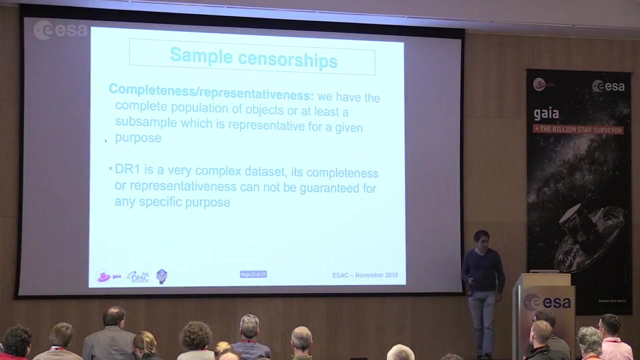 a very positive correlation and here you have a very negative correlation. Take this into account In this release. still, we have problems like this. In future releases, we expect the correlations to be concentrated around zero Censorships. We would like to have a complete. 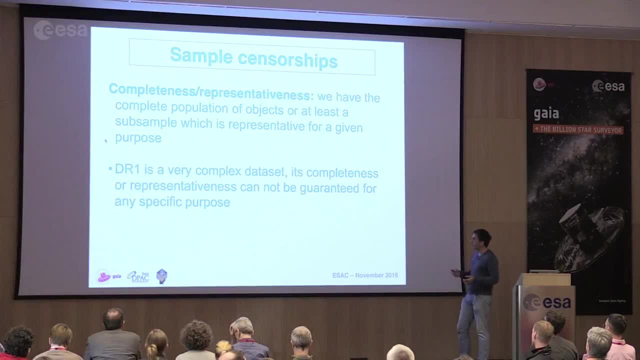 sample, or at least a representative sample, for a given purpose. What's complete for one purpose might not be for another. DR1 is very complex. as I said has already been mentioned, It has been submitted to several combined censorships. The completeness of representativities. 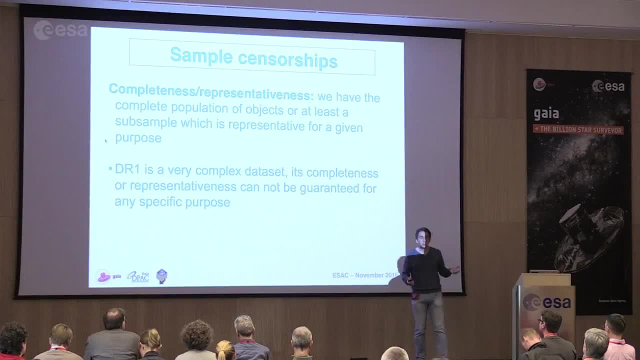 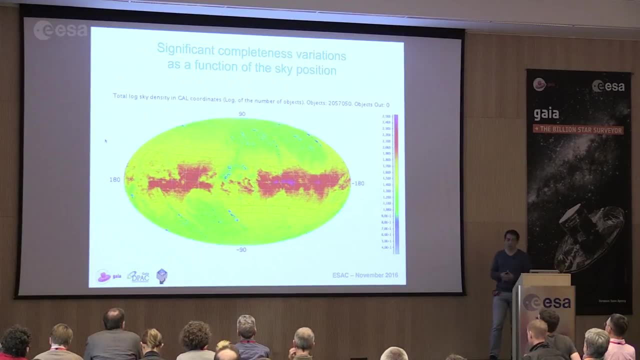 cannot be warranted For any specific purpose. this will improve in DR2.. So be careful when your application of the, when your usage of the Gaia data might depend or might be conditioned by the completeness of the sample. This is the distribution in the sky of the TIGA solution And notice that. 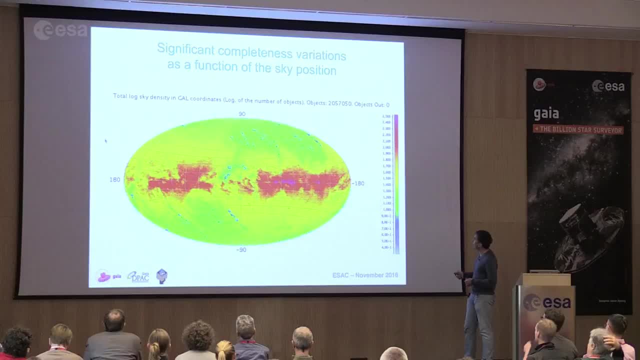 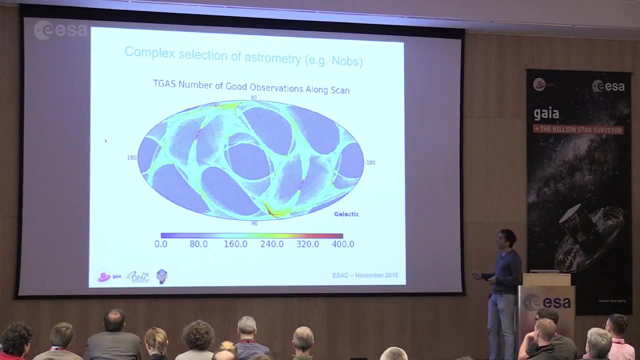 there are strips coming from the scan law and other artifacts. This is the number of good observations of the scan. Since TIGA was selected in part based on the number of good observations. the completeness will be different depending on the region in this. 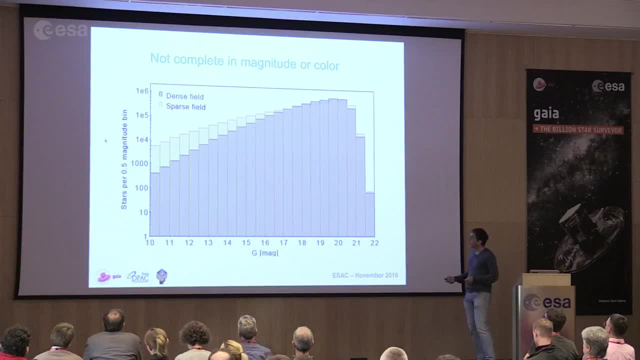 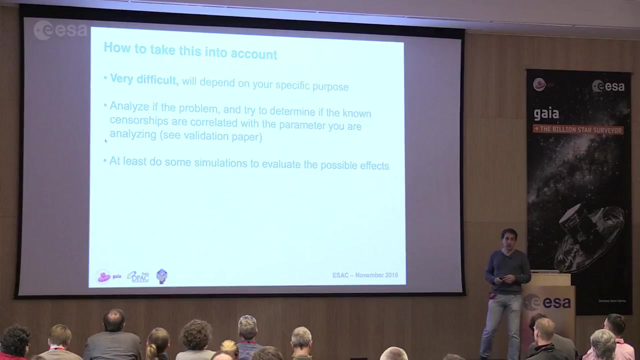 complicated way. This is another example. Due to effects of crowding, the completeness in a dense field might be different than the completeness in a sparse field, et cetera. There are many things like that, But the message is it's very difficult to take into account. 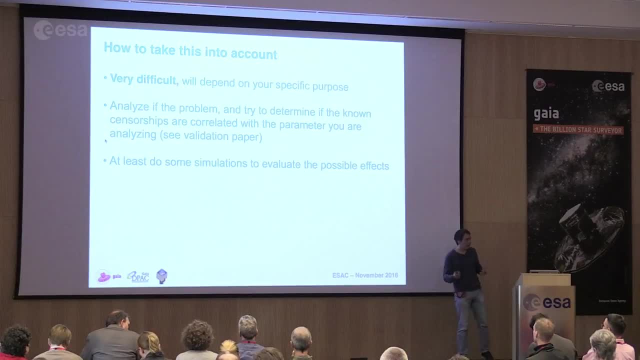 all this, but you at least should have, should be able to take, take into account all this, try to take this, estimate the effect of this incompleteness for your problem, for instance, at least doing some simulations. but, most important, do not make things worse by adding your 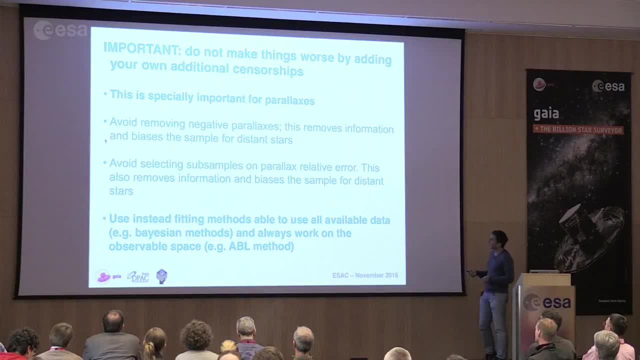 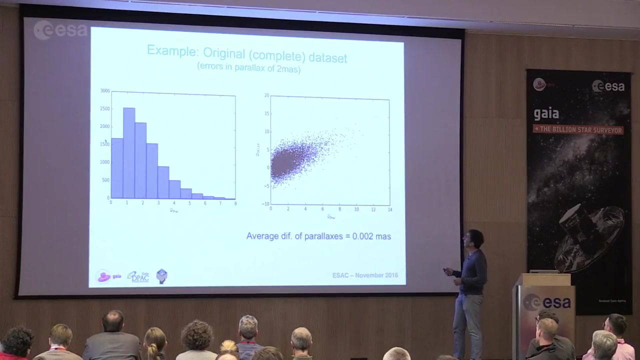 additional sensorships, like removing negative parallaxes or selecting samples, subsamples, on relative parallax error, and always use fitting methods able to use all available data, like variation methods, and always work in the observable space. an example, quick examples: this is a simulation, a complete data set with errors of 2. 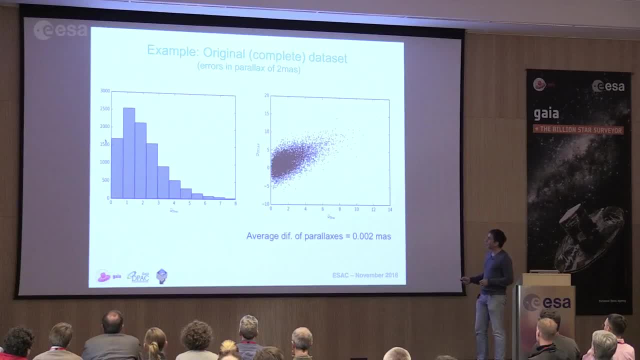 milliac seconds. this is the distribution of the parallaxes of the simulation and this is the true parallax in milliac seconds. with respect to the TIGAs like: well, it's not TIGAs, the errors are a bit large, but TIGAs like. 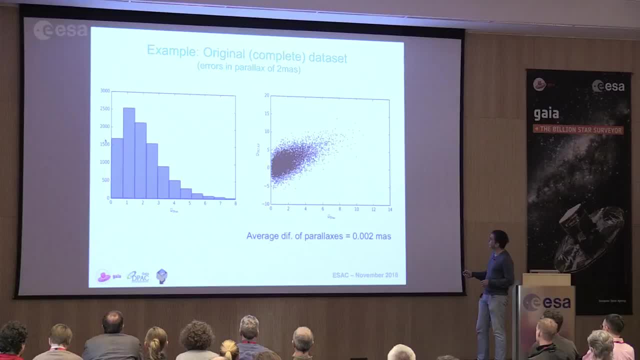 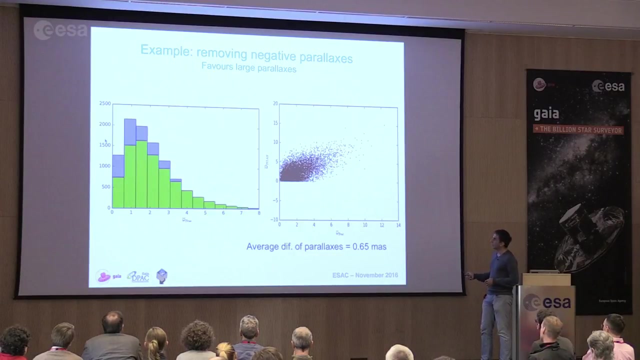 parallaxes. this is the distribution of of true versus of of serve. the average difference of parallaxes is marginal, around zero, because this is the way the sample has been simulated. but if you remove the negative parallaxes first, you are biasing. 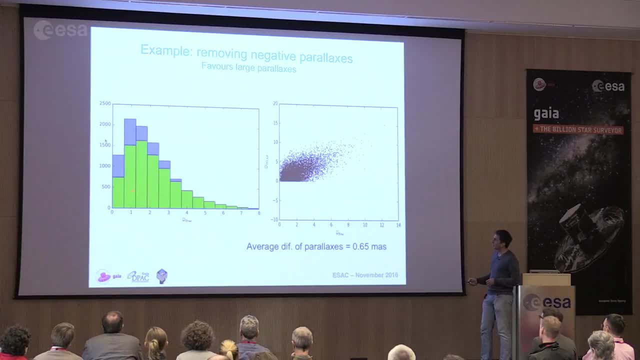 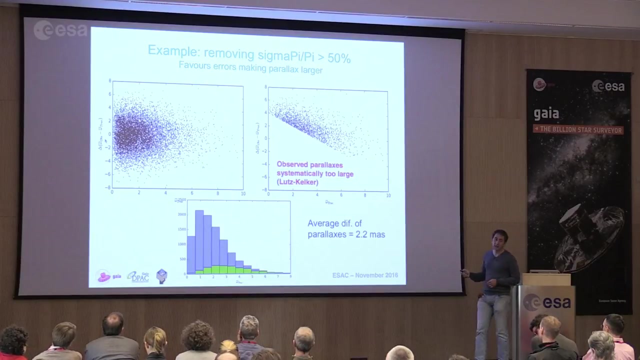 the new distribution of parallaxes, you are removing more small parallaxes than large parallaxes, so now the average difference of parallaxes goes to 0.65 because you have removed a part of the distribution. even worse, if you're remove the parallaxes by a criteria of relative error, like here: 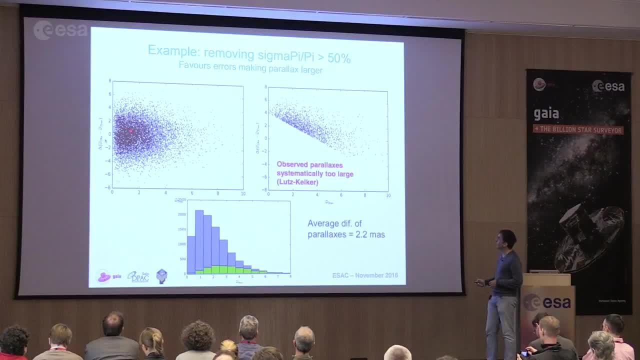 Sigma Pi over Pi larger than 50%. this is what you get with for the complete sample. this is the difference between observed minus true. as a function of the true, you are removing all these parallaxes here. this was us usually known as a Lutz-Skelker bias. so 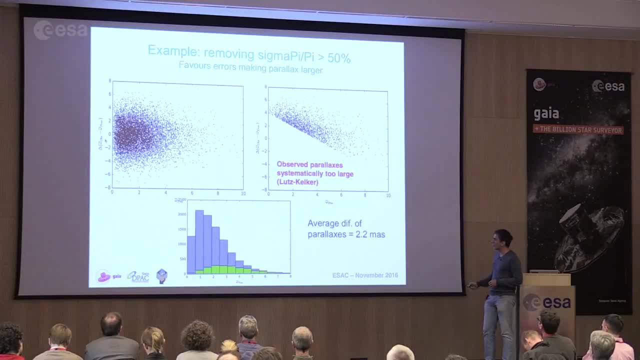 first. you have strongly biased the distribution of parallaxes you want to remove. So you have strongly biased the distribution of parallaxes you want to remove. So you have strongly biased the distribution of parallaxes you want to remove. use Sample and notice that now the average difference of 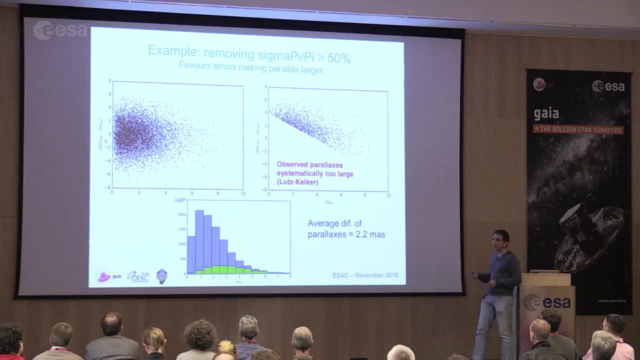 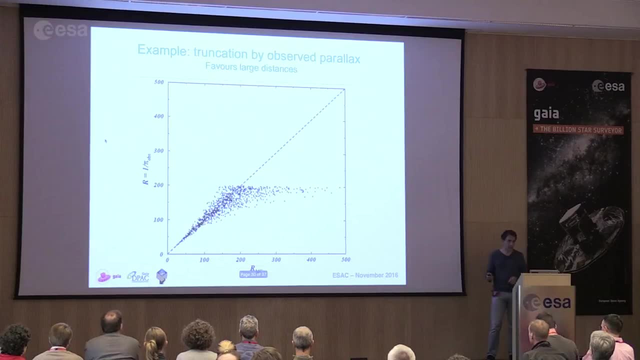 3 verses of serve, 2.2 mass. you have been produced a strong bias in your set of parallaxes, so please do never do that. try to use other methods. another example: if you truncate by observe parallax, this is what happened with the distance. this is another way of. truncate, biasing your sample. more about that in a moment. so me? So, please, please, yes, I hope. then we are ready for our next neural findings. so, please, please. ill also take advantage of these changes. another way of truncating: by observing parralax. this is what happens. this is another way of truncating and biasing your samples. more about that in a moment. but before we will go to the next lesson with graphic theory, 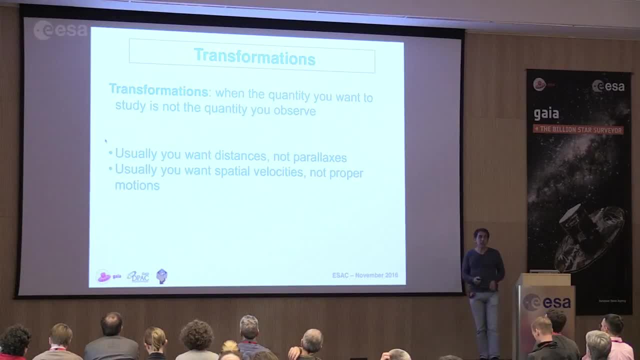 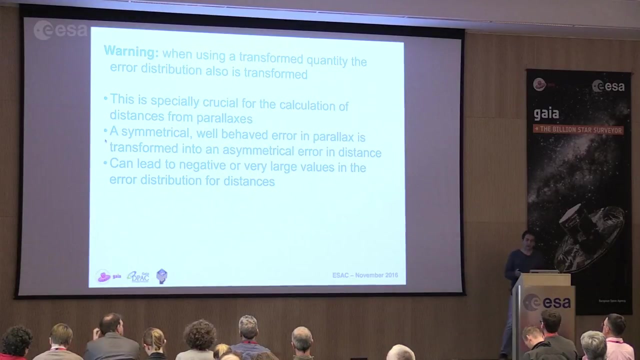 Truncating. This is related to transformations. If you are using or you need a quantity which is not directly observable, like the distance, but instead you are observing another quantity that parallax, there is a transformation involved. A transformation is a bit of a problem because the transformation may change the behavior of the distribution of the errors in your quantity. 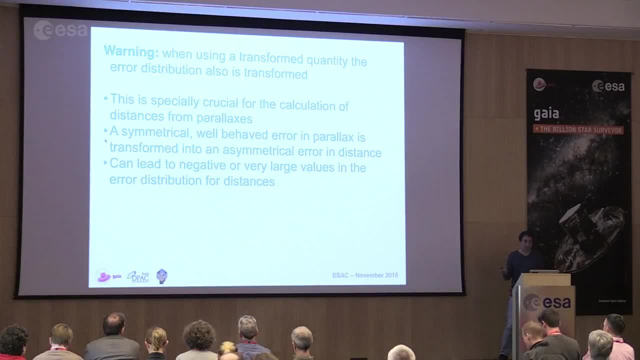 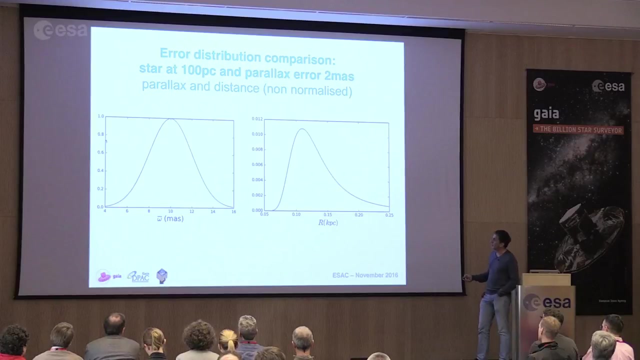 For instance, a well-behaved symmetrical error in parallax might lead to an asymmetrical error in distance. It can lead to negative or very large values due to the shape of the distribution. This is a well-behaved distribution in parallax and this is the corresponding, the matching distribution of errors in distance. 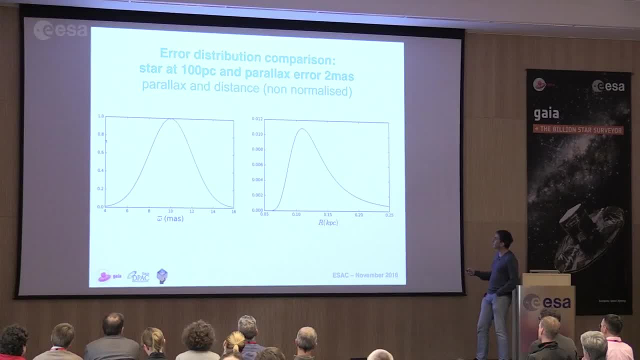 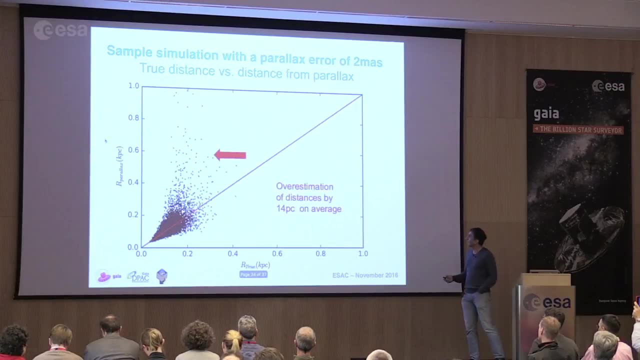 Notice at first, that mode has slightly moved from the true value. The shape is asymmetrical and there is a long tail towards large distances. This is what happens when you compare the true distance from a simulation versus the inversion 1 over pi. This is the result of the tail here. 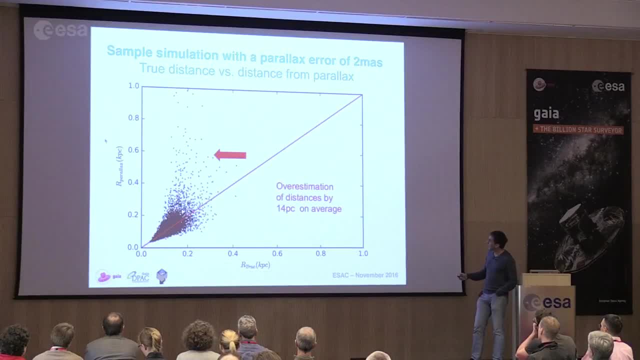 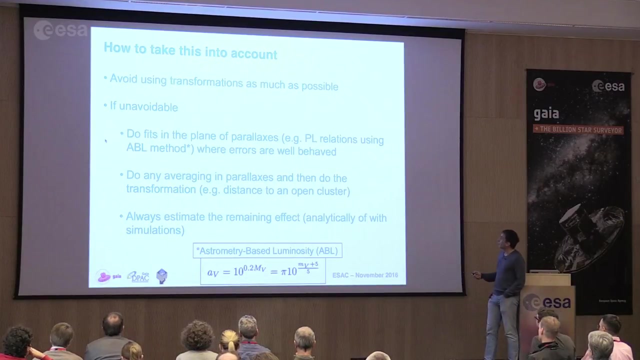 So the distances, just by the fact that you have transformed from parallax to distance, are overestimated on average by 14 parsecs. Just the transformation gives you that. So how to take this into account? Avoid using transformations, if possible. 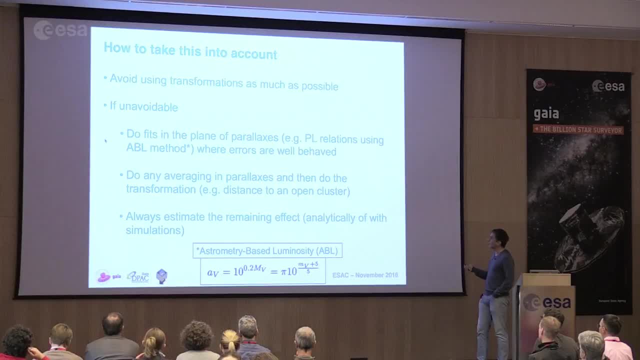 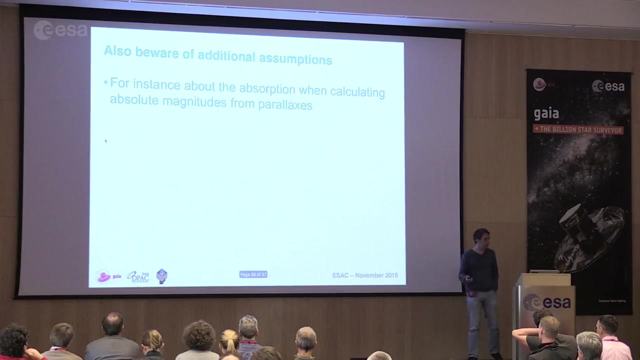 If not possible, use methods like AVM method or Bayesian method that take into account all these effects in a natural way and provide unbiased estimates And, if possible, always estimate the remaining effect that might be there, And, even worse, if you have additional assumptions about, for instance, about absorption. 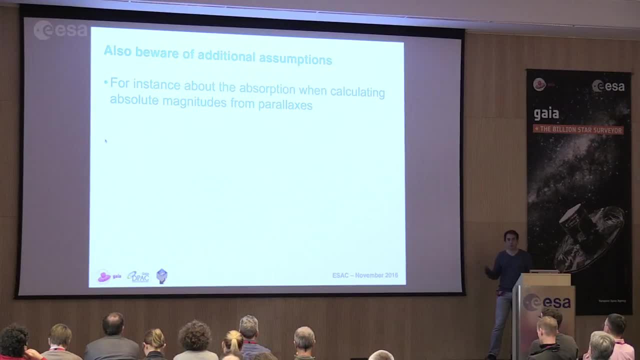 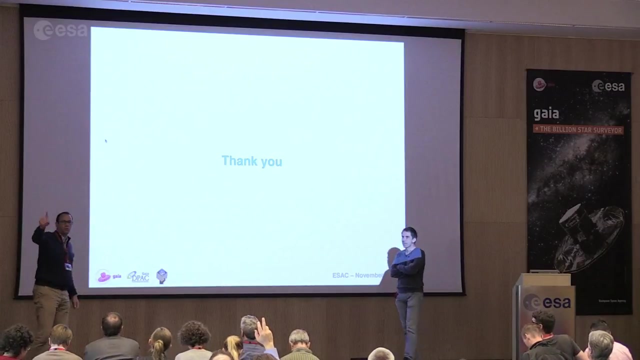 make sure that you put also these kind of assumptions or additional constraints into your Bayesian model, into your method for fitting. Thank you, One or two quick questions and then leave the rest for the discussion this afternoon. Yeah, can you go back to one of your earlier slides? 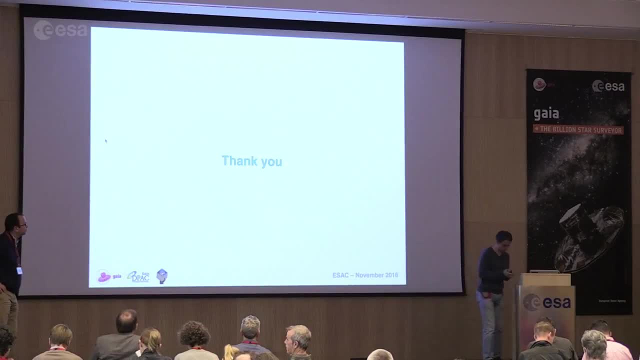 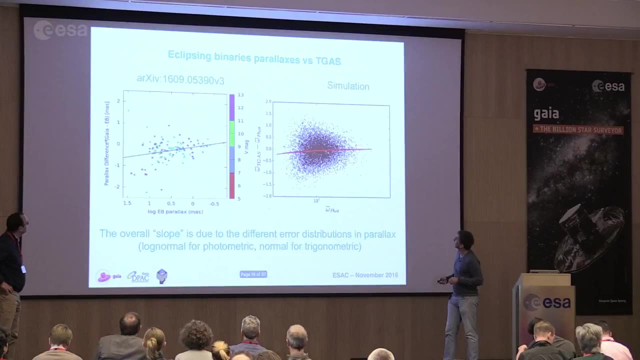 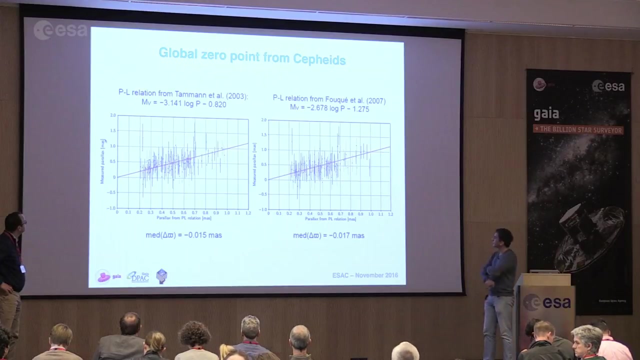 You showed Cepheids as a test And I just had one question to ask you about those. I think it was very early, Much earlier There. So here's an example- And you know, maybe this is similar to what we found- where most of the points go through the error bars. 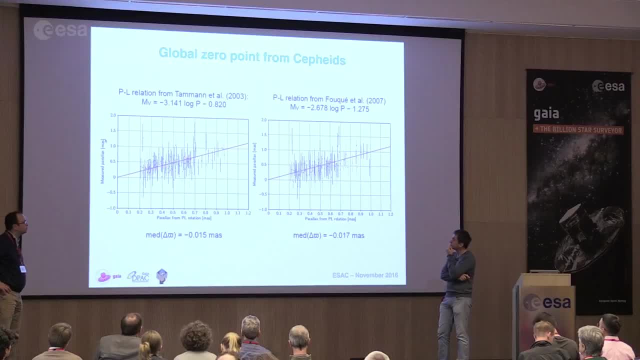 And these are only random errors that you plotted. So what is your reaction to that I mean you talk about? there must be at least a large systematic error. in addition, But how would you like, on the plot on the right there, how would you interpret the too-good chi-square? 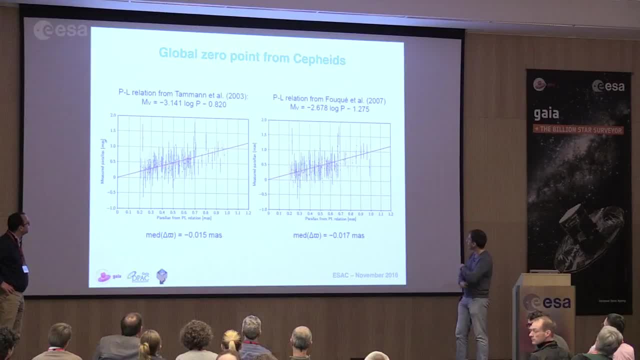 Sorry, I'm not sure I get the. The chi-square is too good in general. It's too good for a plot like this on the right, And you've only included random errors. So how does that leave room for a systematic error? 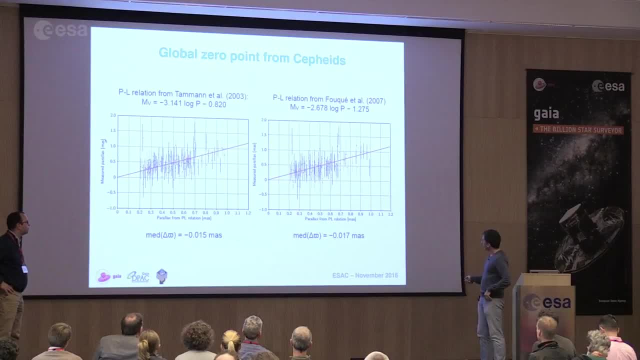 Or how do you interpret it? Okay, This is part of the validation And this is distributed over all the sky, And this would correspond to the zero global zero point, which is estimated at minus .04.. So this should be compared to the minus .04 that we get from validation. 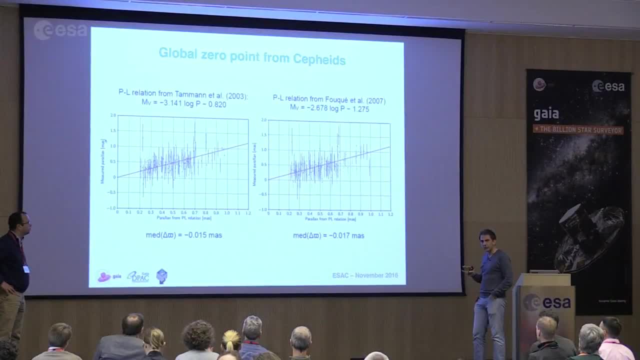 Not to the random variations of all the sky. You see my point. Yeah, but I'm saying: why is the chi-square so good? The error bars go through the line, Yeah, Too good. It's not a one sigma, obviously, somehow. 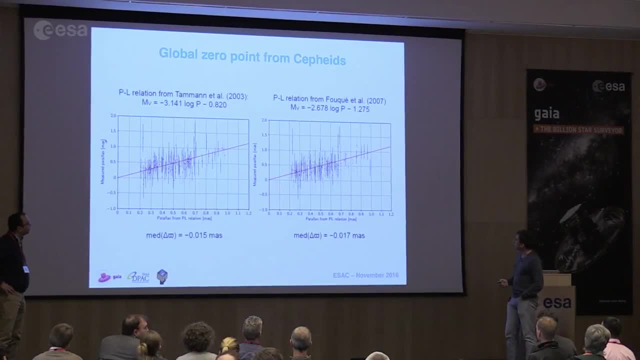 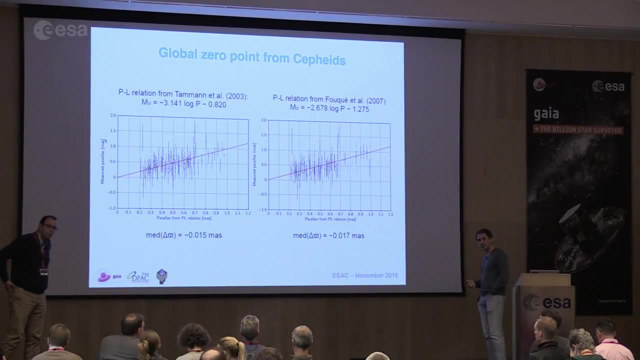 You mean that the fit is too good? Yes, And that's just random errors that you plotted. So I'm getting back to this issue of You're saying the correct errors are the random errors plus the systematic error that you should add. 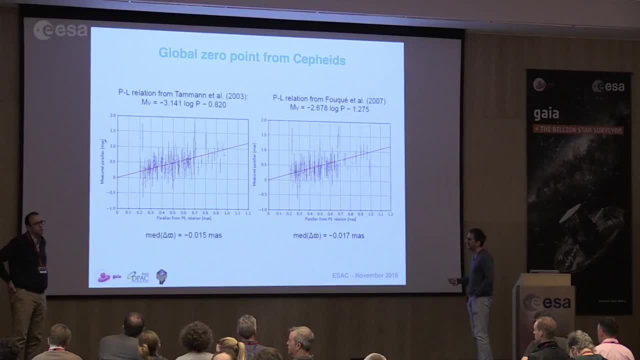 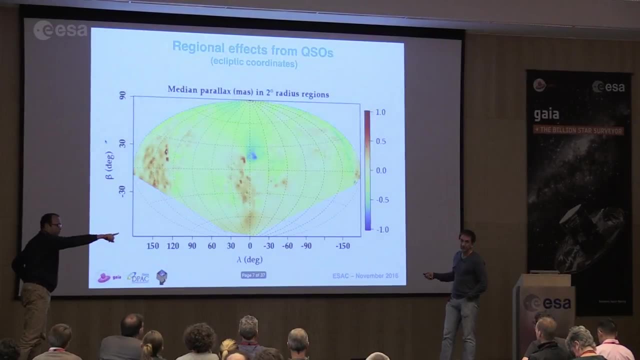 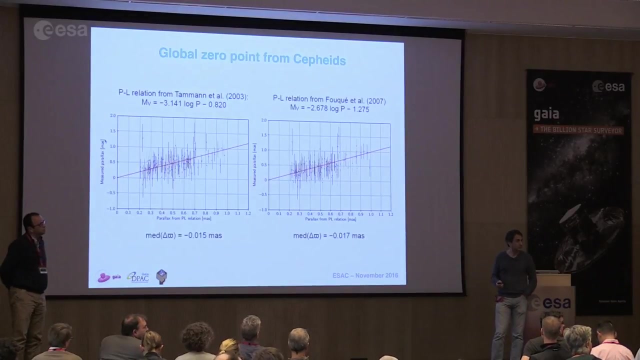 And already it's too good without the systematic error. What do you think? Well, first, we have been overcautious, But you have also to take into account a figure like this, Sorry. Yes, I think this is an interesting question which has a long answer. 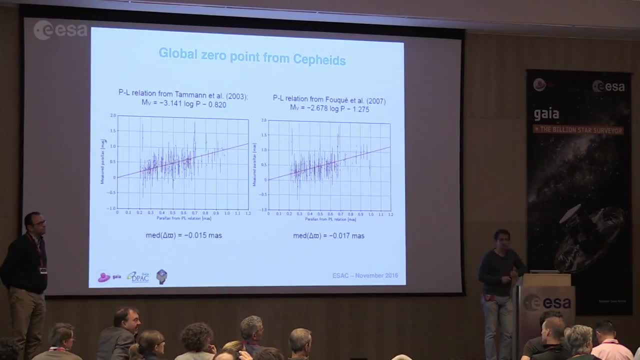 And I suggest that we take that up in the afternoon session. Okay, Yeah, Okay, Take one more. I'm going to put it to the coffee, So you may have said that. Apologies if I missed it, But the plot I guess two slides down from this one where you show. 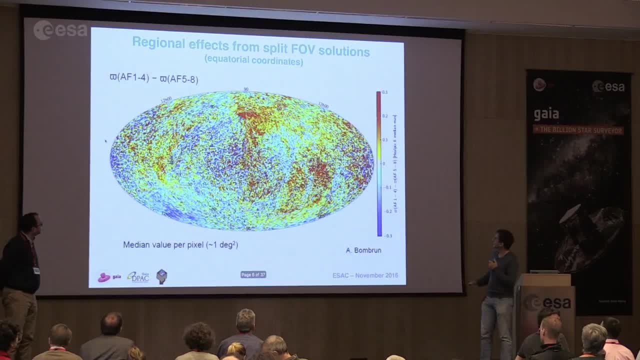 That one, No previous one, Where you show these regional effects. So do you understand? why is there a spatial structure in here? Where does the spatial structure come from? Yes, Okay, If this is just a solution from one half of the focal plane versus another half of. 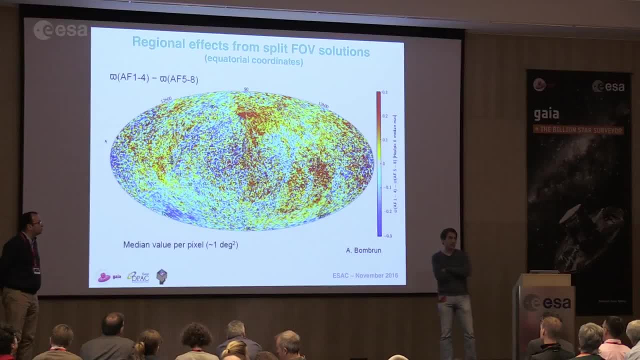 the focal plane, A combination of many factors. The scan load, for instance, is not homogeneous. You have more observations in certain regions than in others, The fitting of the attitude might be worse in some places than in others, et cetera. 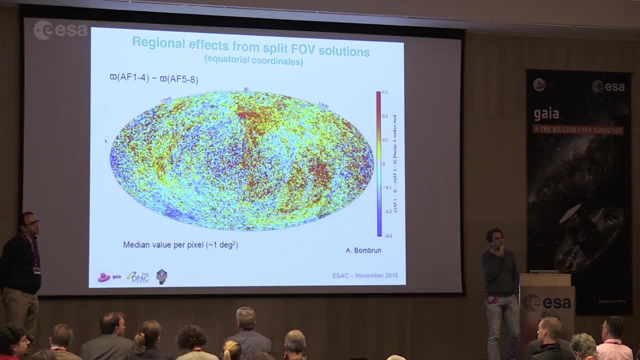 et cetera. So this, But would you expect that to equally affect both parts of the field, Parts of the focal plane? I guess I'm No. This specific one is- I thought you were talking about regional effects- But chromaticity is not affecting both focal planes in the same way. 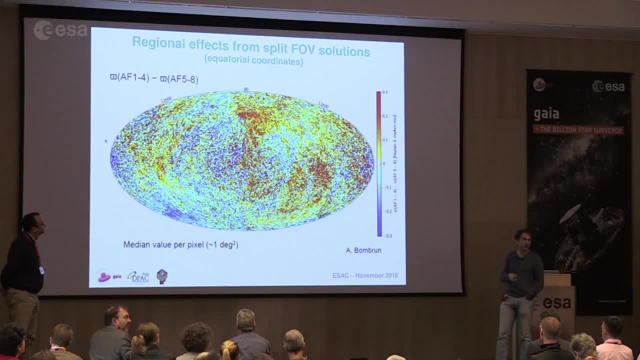 Leonard showed a figure about the chromaticity That this has not been corrected, So the difference can come from this, But I'm not sure I'm getting the question: Why does early versus late depend on where it's coming from? I'm not sure. 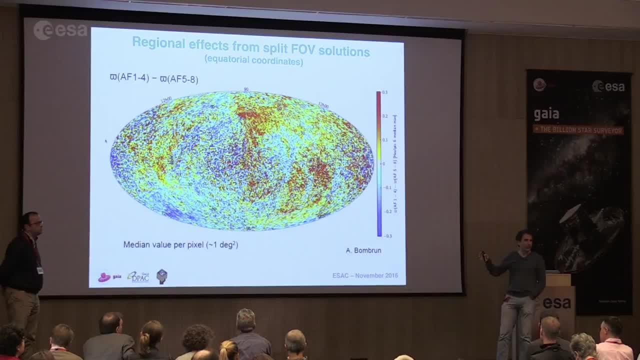